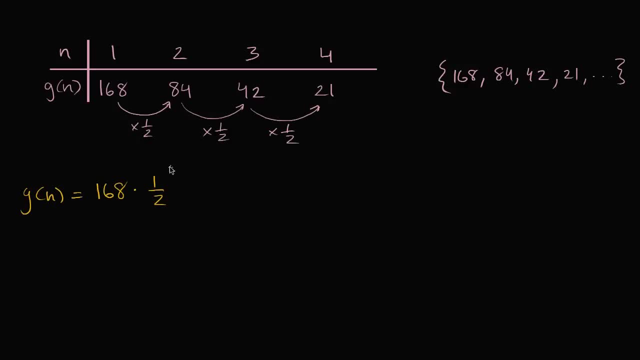 we're gonna multiply by 1 1⁄2 a certain number of times. So we could view the exponent as the number of times we multiply by 1 1⁄2, and how many times are we gonna multiply by 1 1⁄2?? 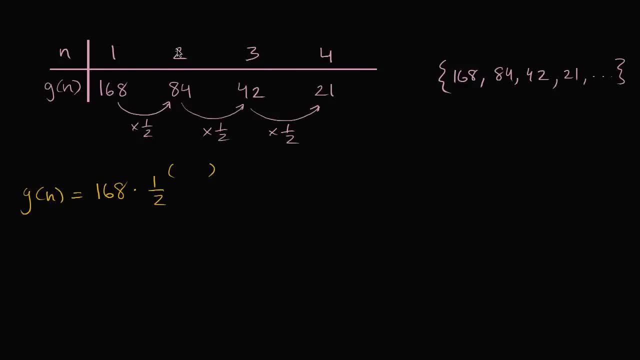 The first term: we multiply by 1 1⁄2 zero times. The second term: we multiply by 1 1⁄2 one time. Third term: we multiply by 1 1⁄2 two times. Fourth term: we multiply by 1 1⁄2 three times. 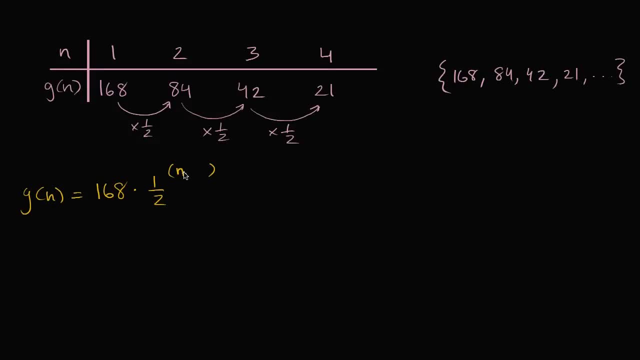 So figure: it seems like whatever term we're on, we're multiplying by 1, 1⁄2 that term minus one times, And you can see that this works. If n is equal to one, you're going to have one minus one. 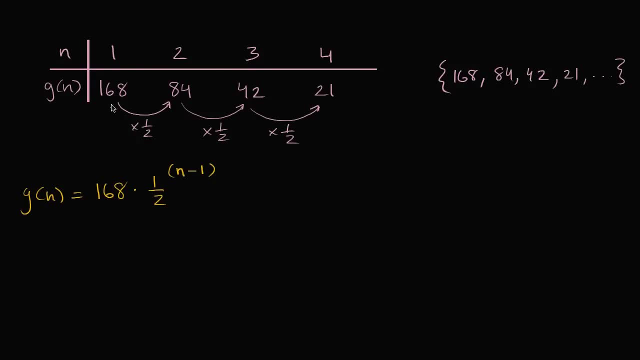 that's just gonna be zero. 1 1⁄2 to the zero is just one, so you're just gonna get a 168.. If n is two, well, two minus one, you're gonna multiply by 1 1⁄2 one time. 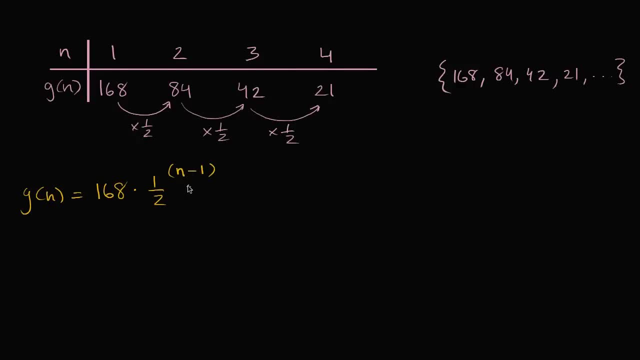 which you see right over here: N is three. you're gonna multiply by 1 1⁄2 twice. n is two is three minus one is two. You're gonna multiply by 1 1⁄2 twice. and you see that right over there. 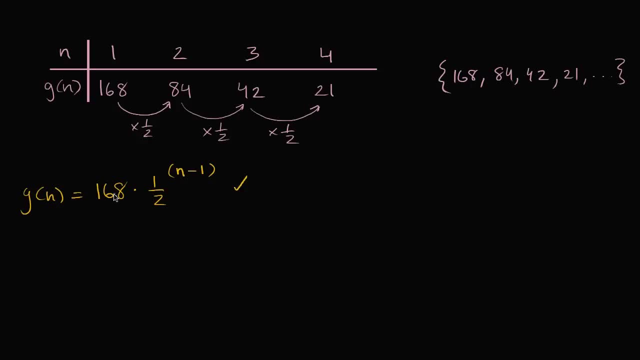 So this feels like a really nice explicit definition for this geometric series, And you could think of it in other ways. You could write this as g of n is equal to. let's see one way you could write it as you could write it as 168,. 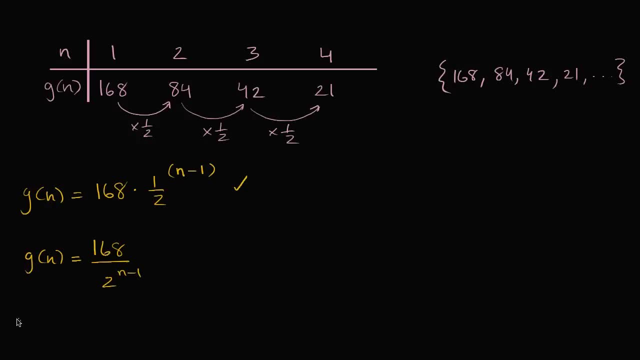 and I'm just algebraically manipulating it over: two to the n minus one. Another way you could think about it is: well, let's use our exponent properties a little bit. We could say: g of n is equal to, let's see: 1: 1⁄2 to the n minus one. 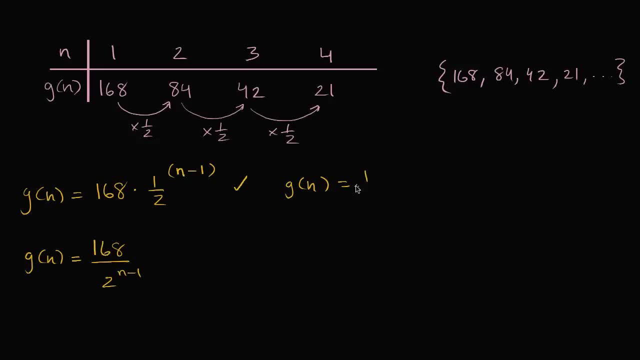 that's the same thing as 1 1⁄2,. let me write this: it's equal to 168,. let me do this in a different color. So this part right over here is the same thing as 1 1⁄2 to the n. 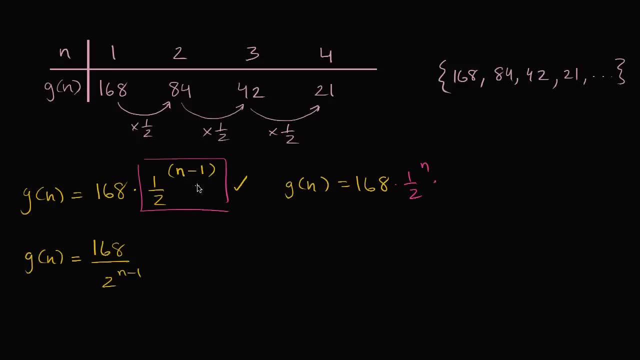 so times 1 1⁄2 to the n, times 1 1⁄2 to the negative one, 1 1⁄2 to the negative one. Well, 1 1⁄2 to the negative one is just two. 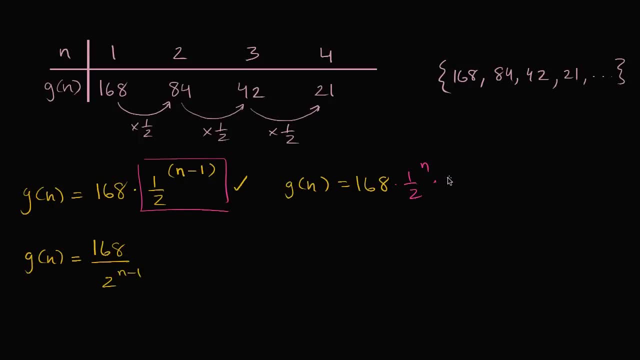 is just two, so this is times two. So we could rewrite this whole thing as: 168 times two, is what? 336? 336, did I do that right? 160 times two would be 320, plus 16,, two times eight. 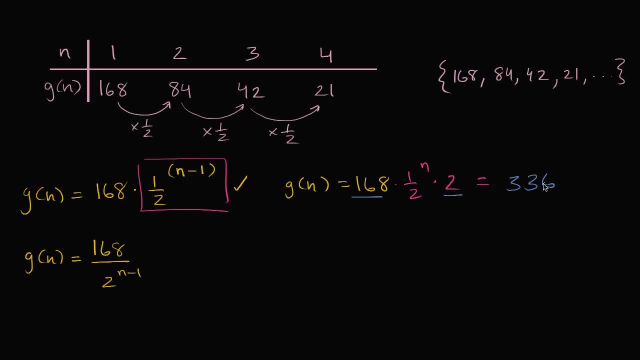 So yeah, 336,. and then times 1 1⁄2 to the n, Times 1 1⁄2 to the n. So these are equivalent statements. This one makes a little bit more intuitive sense. it kind of jumps out at you: you're starting at 168,. 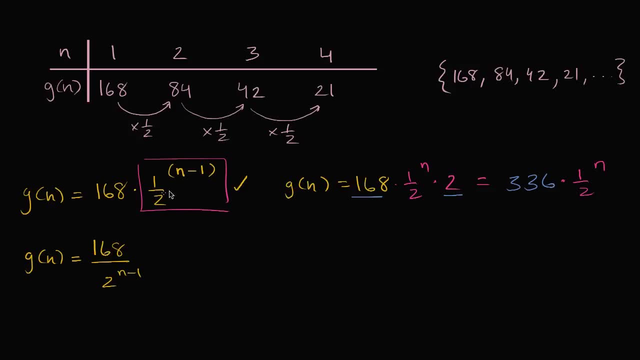 and you're multiplying by 1, 1⁄2, whatever term, you are minus one times, but this is algebraically equivalent to this, to our original one. Now can we also define g of n recursively, And I encourage you to pause the video and try to do that. 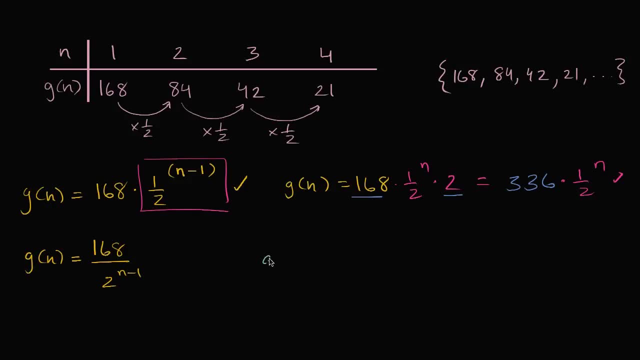 And in a lot of ways the recursive definition is a little bit more straightforward. so let's do that G. well, I'll make the recursive function a different. well, I'll still stick with g of n, Since it's on this table right over here. 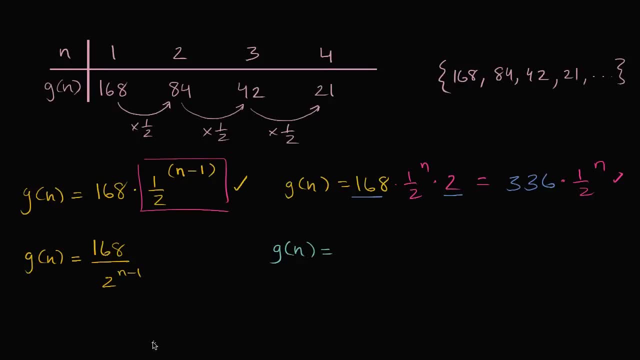 G of n is equal to. so let's see if we're going to when n equals one. if n is equal to one, we're starting at 168, 168.. And if n is greater than one and a whole number. 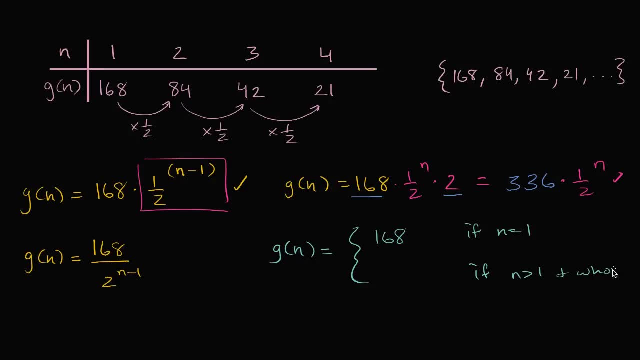 so if n, so this is gonna be defined over all positive integers and whole number. what are we gonna do? Well, we're gonna take 1⁄2 and multiply it times the previous term. So it's gonna be 1⁄2 times g of n minus one. 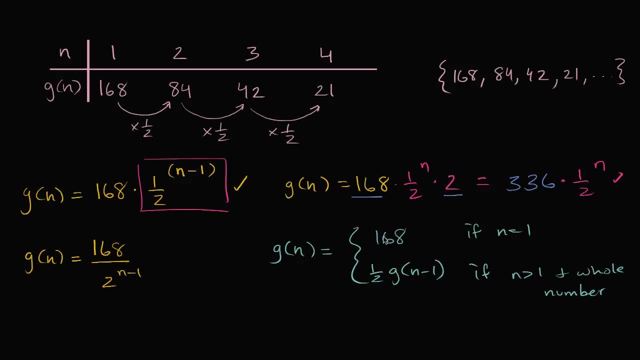 And you can verify that this works. If n is equal to one, we just go right over here. it's gonna be 168.. G of two is gonna be 1⁄2 times g of one, which is of course 168.. 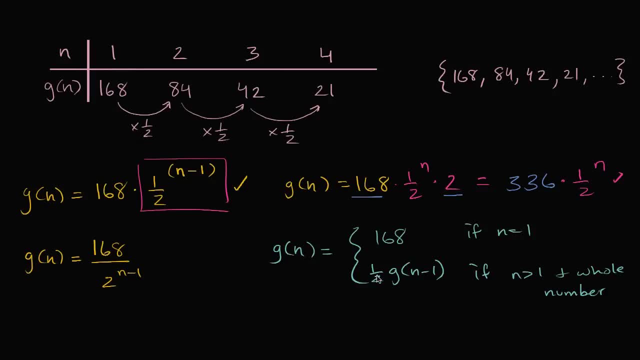 So 168 times 1⁄2 is 84.. G of three is gonna be 1⁄2 times g of two, which it is. G of three is 1⁄2 times g of two, 1⁄2 times g of two. 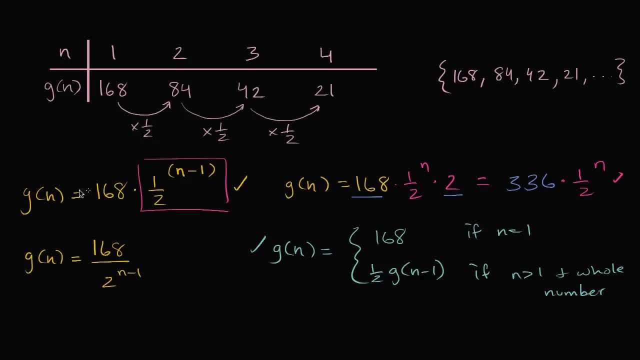 So this is how we would define. this is the explicit definition of this sequence. This is a recursive function to define this sequence.